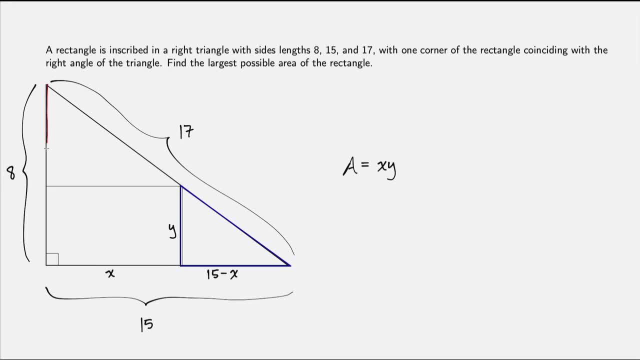 And that triangle right there, is similar to this larger triangle here, And so we're going to go ahead and consider those two And we're going to set up a, a proportion, using similar triangles, in order to find that relationship between x and y. I'm going to take this length down here. 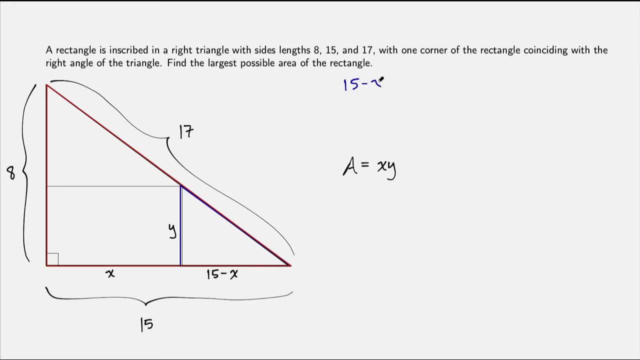 for the smaller triangle We'll take 15 minus x divided by the height of that triangle, y, And that's going to equal. and then for the larger triangle the length down here is 15.. And then that height of that larger triangle is 15.. 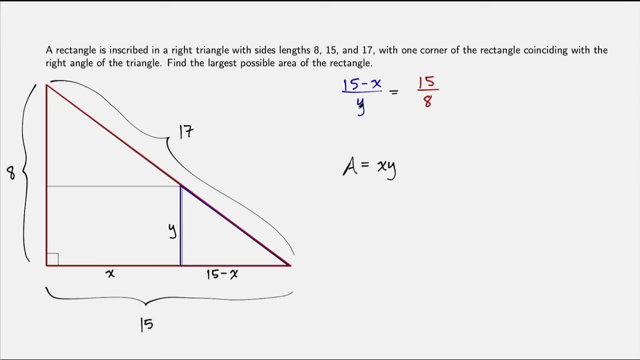 And then that height of that larger triangle is 8.. So there's a relationship that exists between x and y, And so now we can, we can solve for one of those variables. I'm going to go ahead and solve for y. We can start here by cross multiplying. 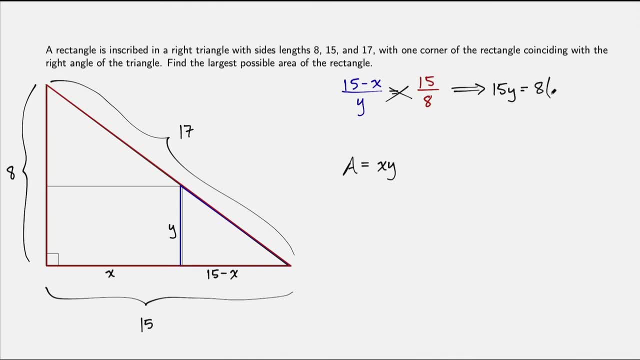 And we get 15y equals 8 times 15 minus x. And then divide both sides here by 15 and get y equals 8 over 15 times 15 minus x. And since that is y, I can now take that and plug it in right here for y. 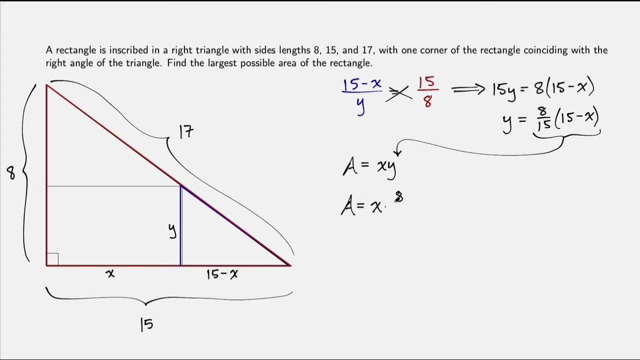 So I get my area is x times 8, over 15 times 15 minus x, And we're looking for the smallest- or sorry, the largest- that this area could possibly be, And so we're going to go ahead and graph this in our calculator. 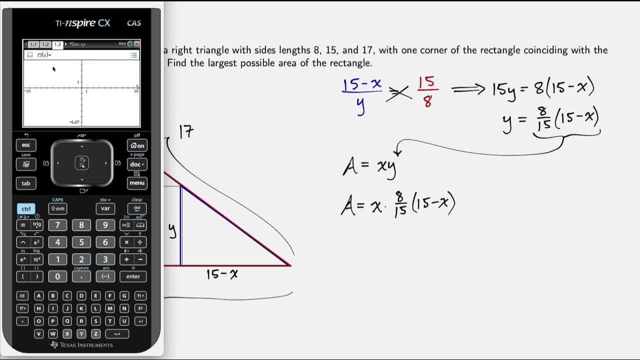 and find that maximum point. So to graph here: we have x times- sorry, I mean x times 8- over 15 times 15 minus x, And we're going to graph it here And we're going to get that maximum point. 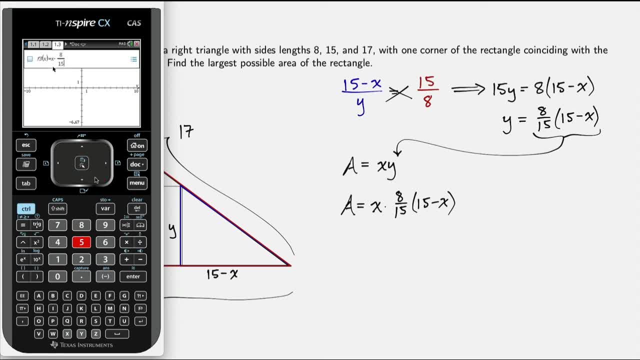 We have x times minus 8.. And we're going to get that maximum point 8 over 15 times 15 minus x. Graph that We're looking for the largest this can be. so we're looking for a maximum. So I'm going to go ahead and zoom out. Oop, that's not what I wanted. 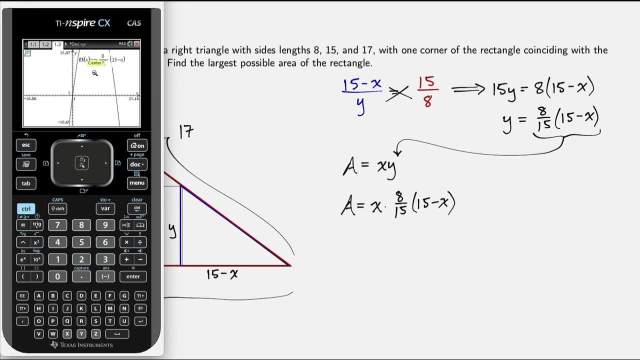 We're going to go ahead and zoom out until we can find that And there's a maximum up there. So we'll go to menu analyze graph and we're going to find that maximum. So we're going to click to the left of that maximum and to the right of that.